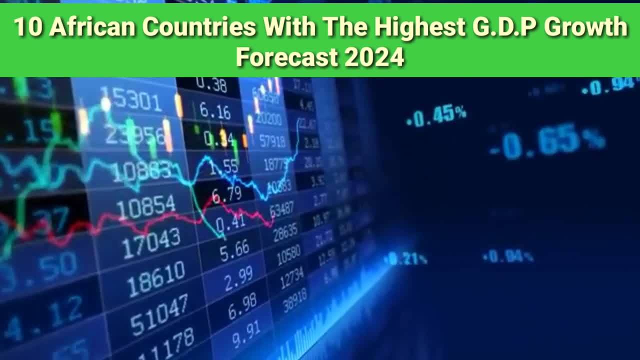 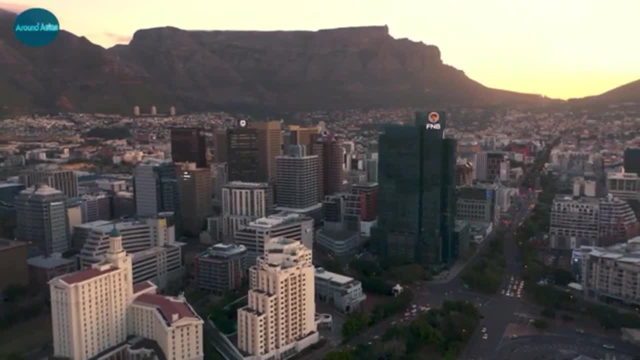 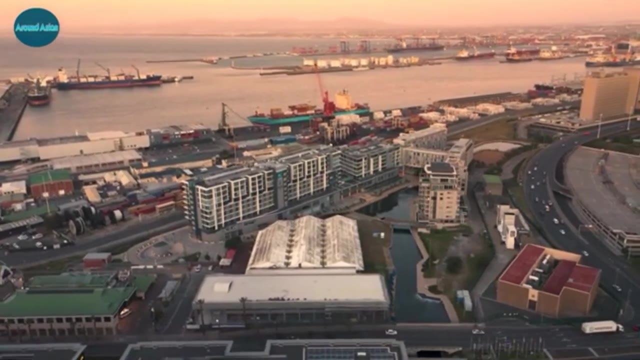 economies with highest GDP growth forecast for 2024.. 10. South Africa: 1.8% growth. South Africa, despite facing economic challenges in recent years, is projected to experience a GDP growth of 1.8%. The country's economic recovery is influenced by factors such as structural reforms. 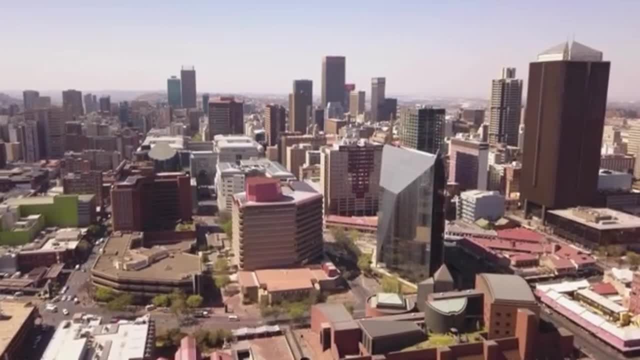 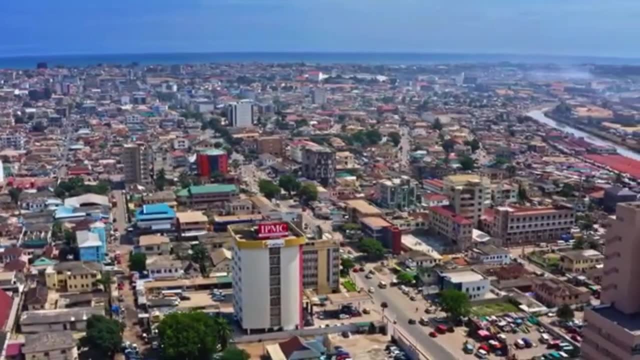 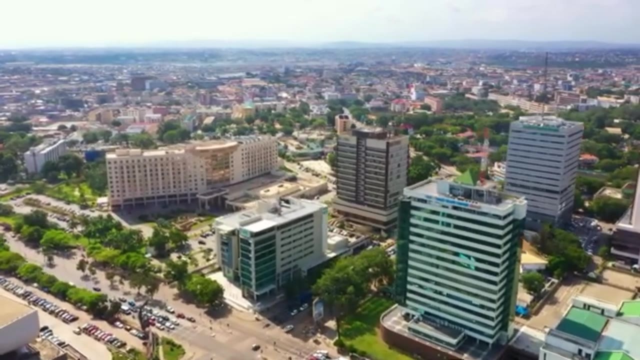 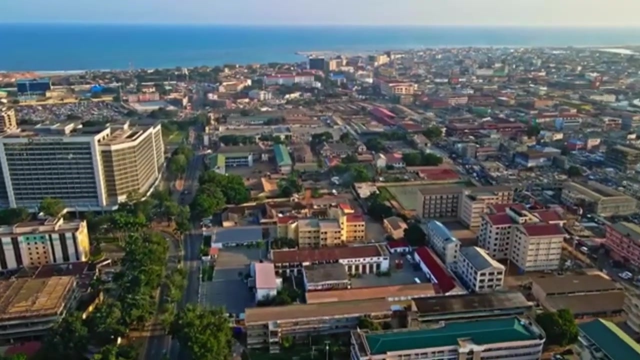 mining sector improvements and efforts to attract foreign investments. 9. Ghana: 2.5% growth. Ghana, a country located in West Africa, is known for its political stability and economic reforms. The country secured the ninth position on this list with a GDP growth forecast of 2.7%. The country's focus on industrialization 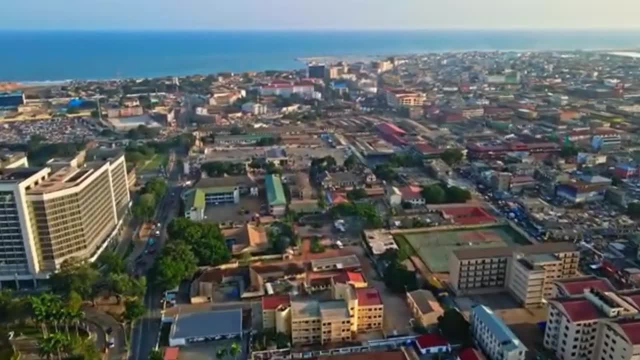 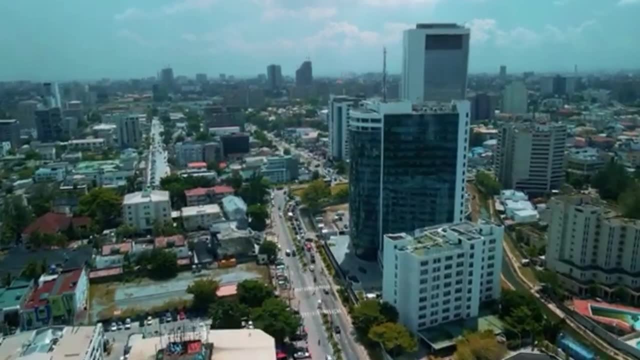 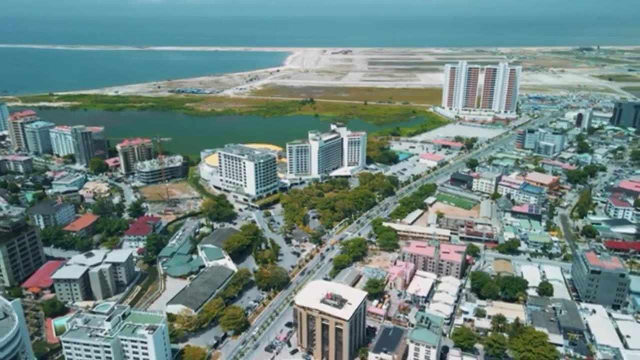 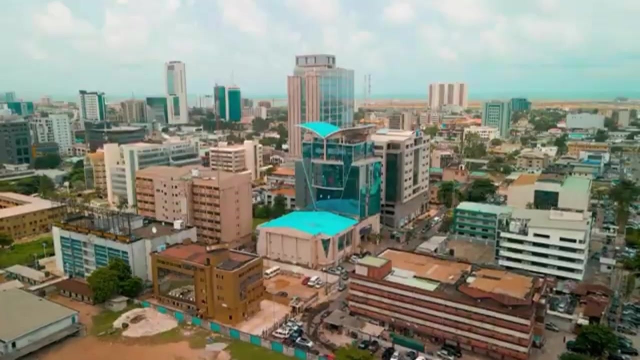 technology and sustainable development positions it for continued economic growth. 8. Nigeria: 3.1% growth. Nigeria, the largest economy in Africa, is projected to experience a GDP growth of 3.1% in 2024.. Following a challenging period, Nigeria's economic diversification efforts and reforms in 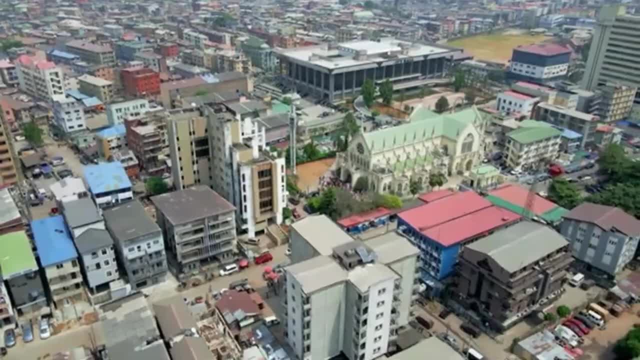 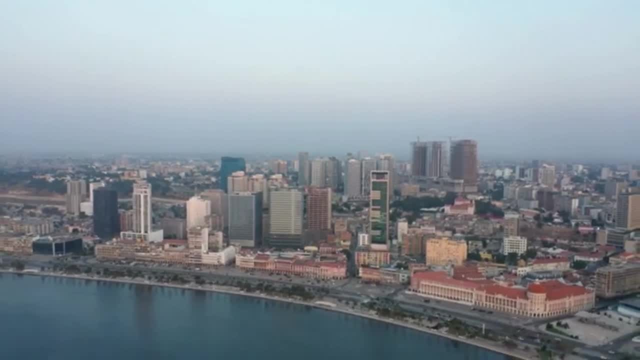 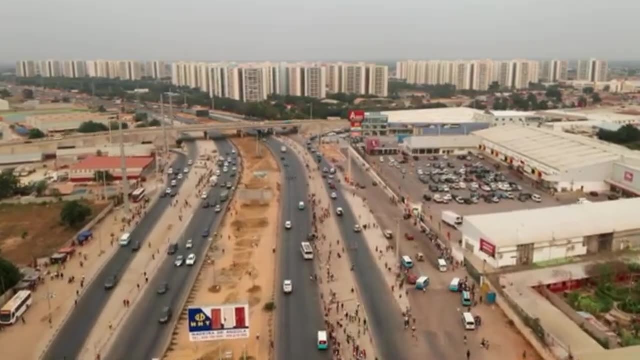 sectors like agriculture and manufacturing contribute to its positive growth forecast. 7. Angola: 3.3% growth. Angola secures the seventh spot with a GDP growth forecast of 1.8%. The country's economic recovery is projected to experience a GDP growth forecast of 3.3%. The country's oil-dependent economy has 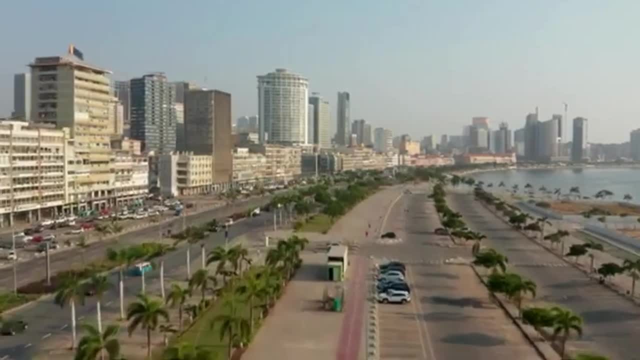 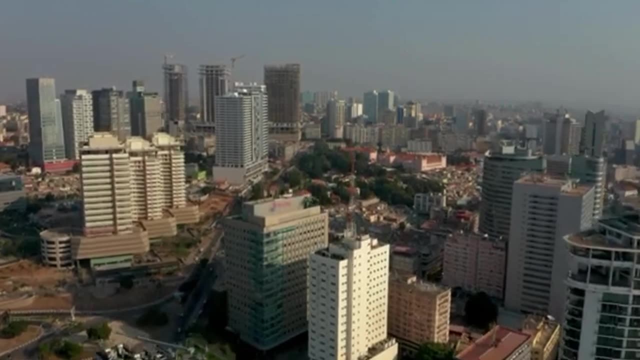 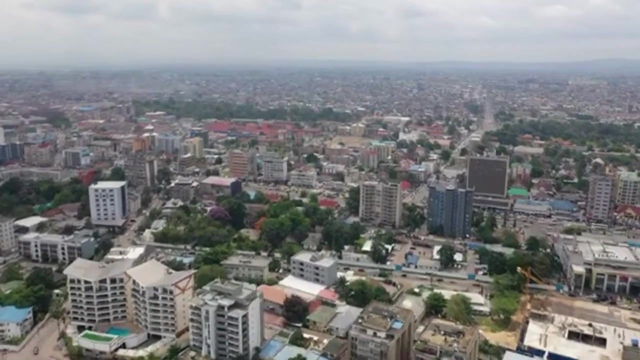 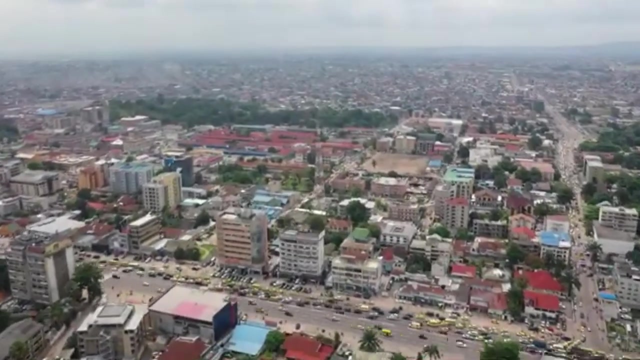 been diversifying into sectors like agriculture and mining. Ongoing economic reforms and efforts to improve the business environment contribute to Angola's positive economic outlook. 6. DR Congo: 4.7% growth. The Democratic Republic of the Congo, with a GDP growth forecast of 4.7% reflects the potential of this vast and resource-rich 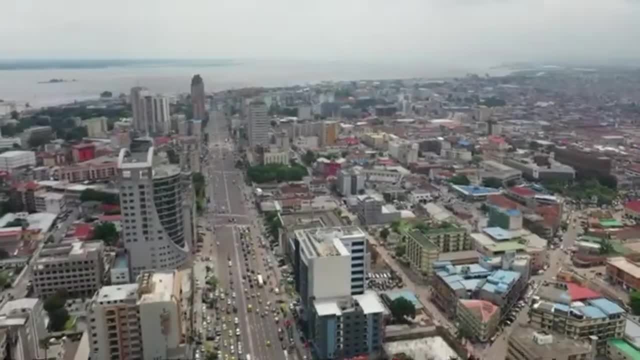 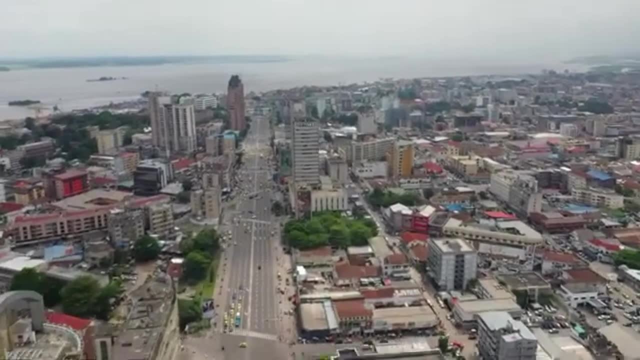 blows Caribbean residents on to a standing modern market. In 2007,, the study revealed the ability of a country to boost finance and parallel engineering fuerak in a rich nation, Despite challenges related to governance and infrastructure. the DRC's wealth in natural resources, including minerals and agriculture, positions it for economic expansion with strategic investments and reforms. 5. Kenya- 5.3% growth. Kenya, a key player in East Africa, secures the fifth position with a GDP growth forecast of 5.3%. 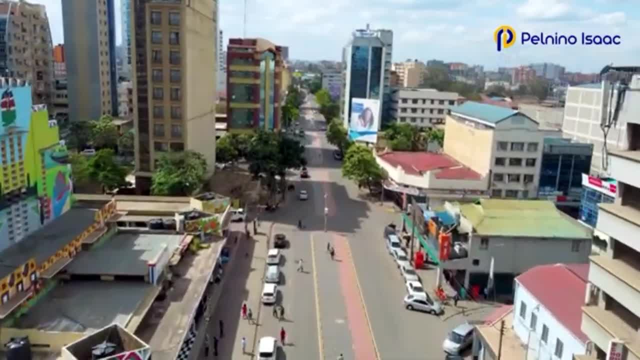 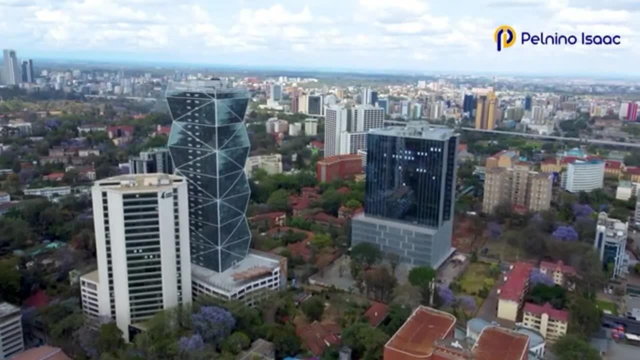 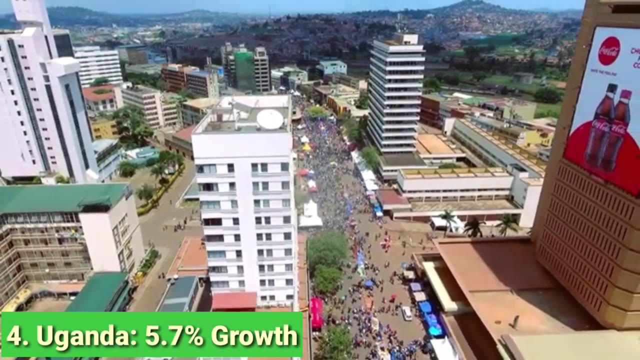 economy, technology, innovation and strategic geographic location contribute to its economic strength. Government initiatives such as Big Four Agenda further support Kenya's growth trajectory and the newly implemented Kenya Vision 2030.. 4. Uganda: 5.7% Growth.